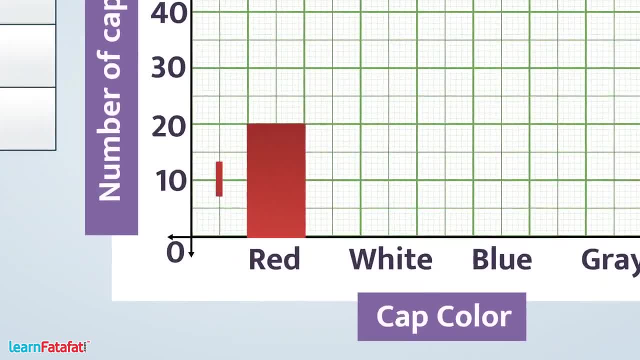 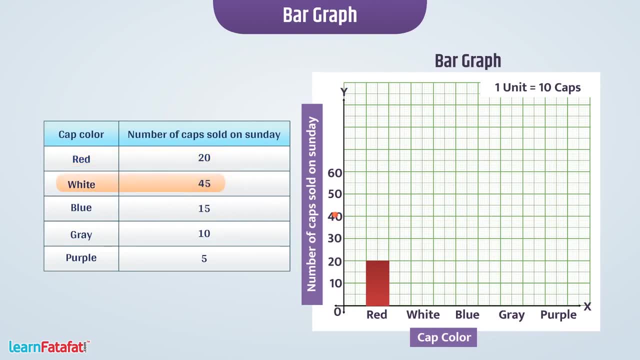 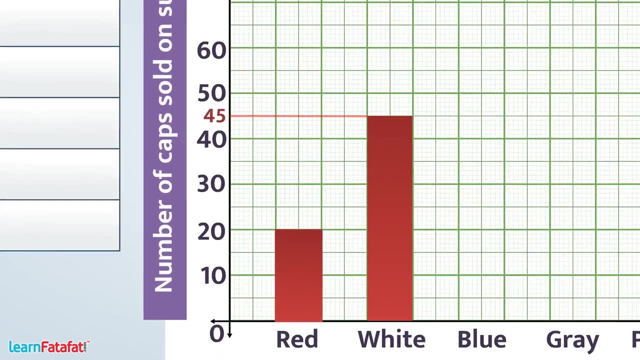 on vertical axis It will be a bar of height 2 units. Similarly, for representing 45 white caps, we draw a bar extending from 0 to 45 on vertical axis. Here note that any two divisions have 10 subdivisions. 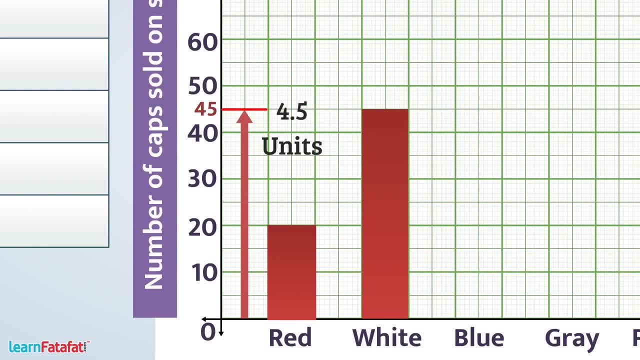 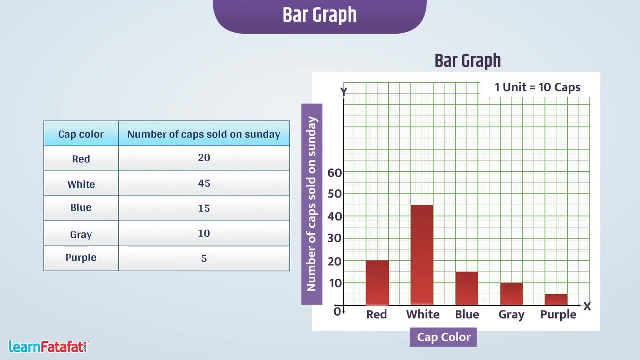 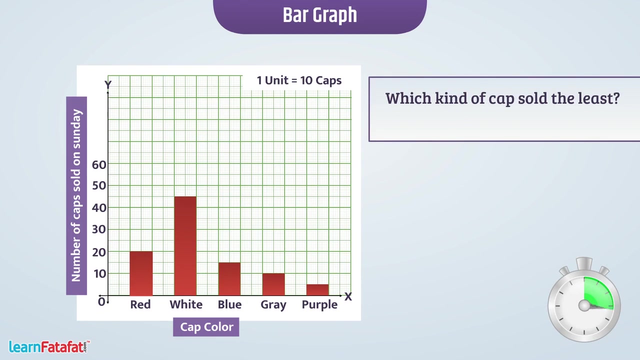 So 45 will be represented by 4.5 units. This is how we can represent all the data on the bar graph. The advantage of bar graph is we can represent data much easily as well as in less time. By looking at bar graph, can you tell me the kind of caps sold the least? 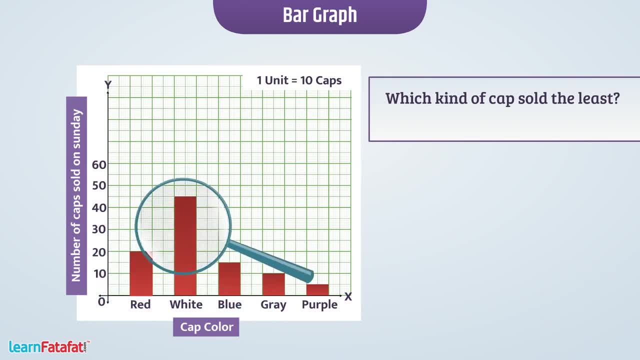 Here, the bar with the smallest height will be the answer. So purple colored caps are sold the least. Can you tell me what is the difference between the number of red caps and blue caps? We can see that the height of bars differ by half unit. 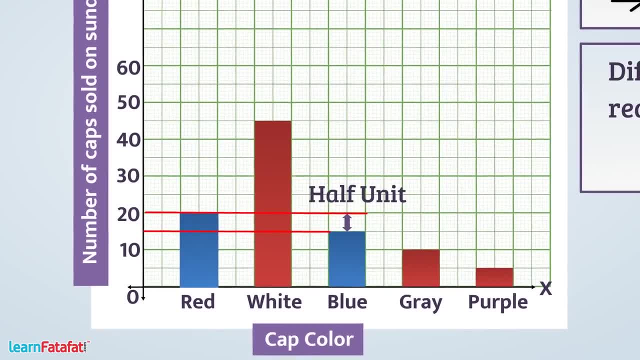 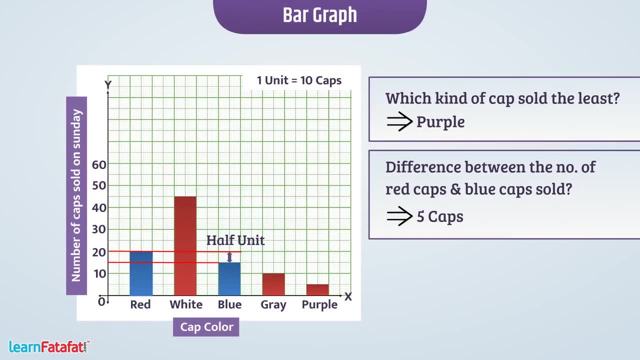 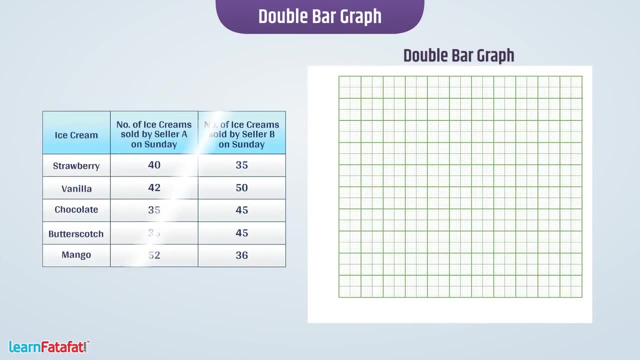 Since one unit represents 10 caps, so we can say that half unit represents 5 caps. Now let's understand more about double bar graph. Following table shows the number of ice creams sold by seller A and seller B on Sunday. The number of ice creams sold by seller A and seller B on Sunday. 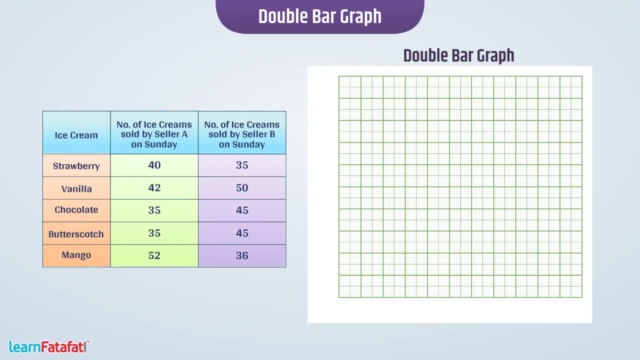 Thanks for watching. To draw a double bar graph: observe the values. We can see that lowest value is 35 and highest value is 52.. To draw a double bar graph: observe the values Here: if we use 1 unit is equal to 1 ice cream, then the bars will be very tall and we could not represent them on the paper. 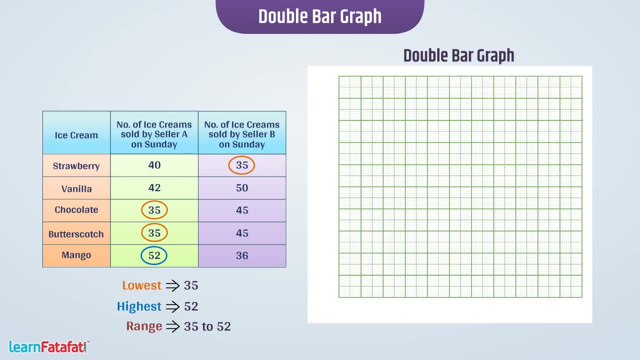 Here. if we use 1 unit is equal to 1 ice cream, then the bars will be very tall and we could not represent them on the paper. use a very large value, such as 1 unit is equal to 50, then it will be difficult to. 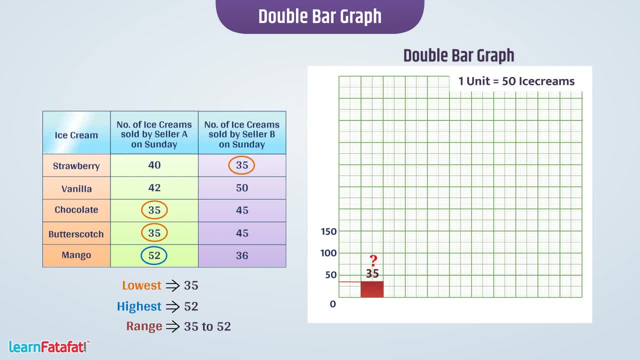 represent values like 35, so an appropriate scale could be: 1 unit is equal to 5 ice creams or 1 unit is equal to 10 ice creams, as most of the value can be represented using this key. can we choose 13 here? think about it. 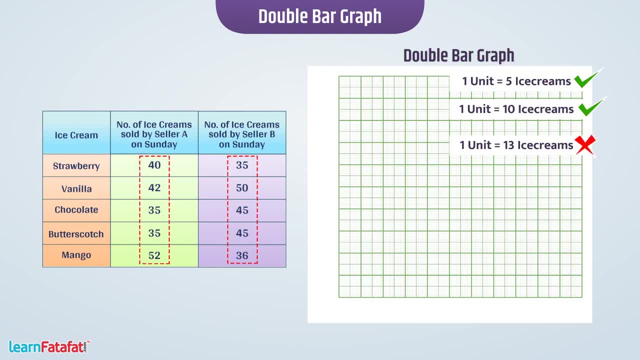 no, since given values are not multiple of 13 or they cannot be easily represented. therefore, we cannot take 13 as the value of unit length. we will choose 1. unit length is equal to 10 ice creams. now here we have to draw two bars, so we must differentiate them so that we can read them easily. 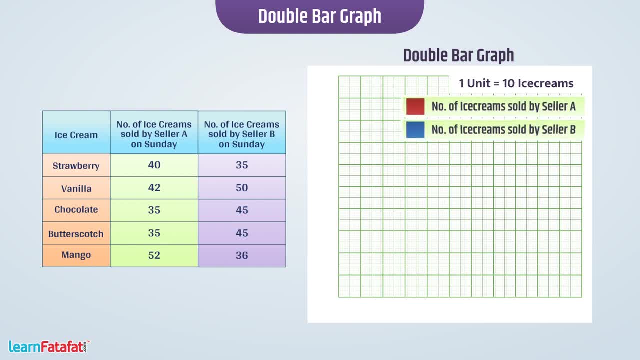 to do so. we can write legends like this. we can draw bar like this to show the number of ice creams sold by seller a on Sunday and bar like this to show the number of ice creams sold by seller B on Sunday. let's draw the double bar graph. first, draw vertical and horizontal axis. 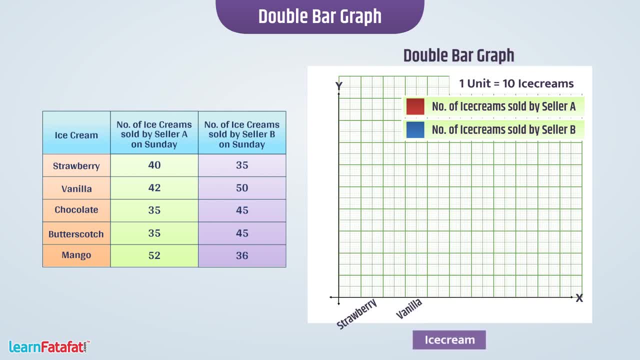 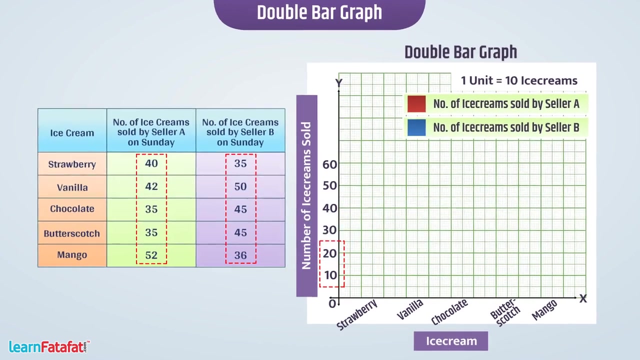 show categories like strawberry, vanilla, chocolate, etc. on horizontal or vertical axis and show number of ice creams on other axis, according to the scale taken here, since value less than 30 are not present, so we can skip those values and can start from 30 as well. to do so, we will draw a kink. 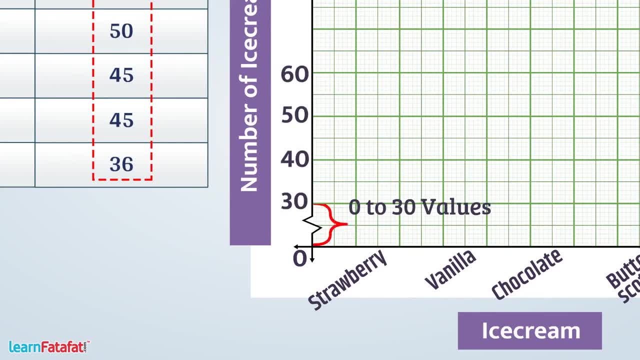 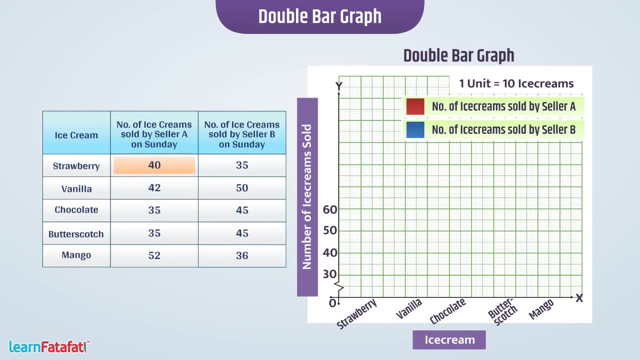 mark which shows that the values from zero to thirty are not taken. seller a sold 40 strawberry ice creams, so we will draw bars of length 0 to 40. he sold 42 vanilla ice cream, so we will draw bars of length 0 to 40. 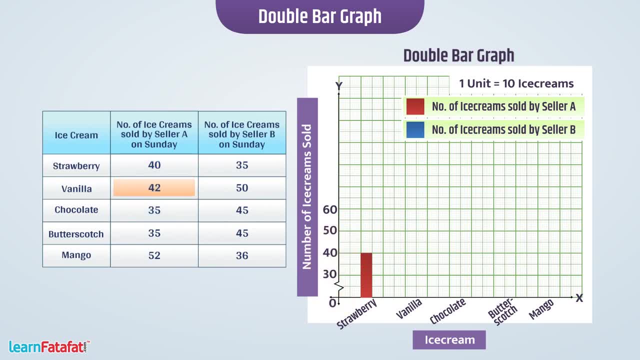 he sold 42 vanilla ice cream, so we will draw bars of length 0 to 40. Here, 42 is between 40 and 50.. Since each unit represents 10 ice creams, therefore we can say that the 10th part of unit represents 1 ice cream. 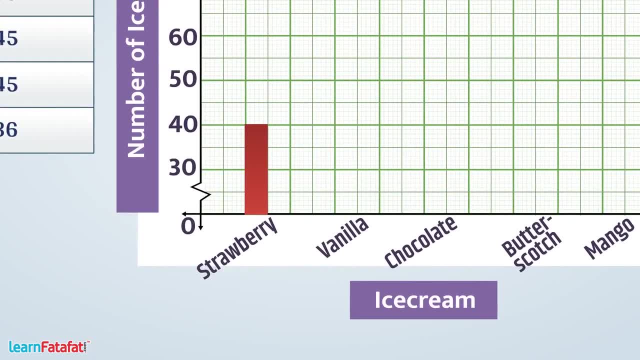 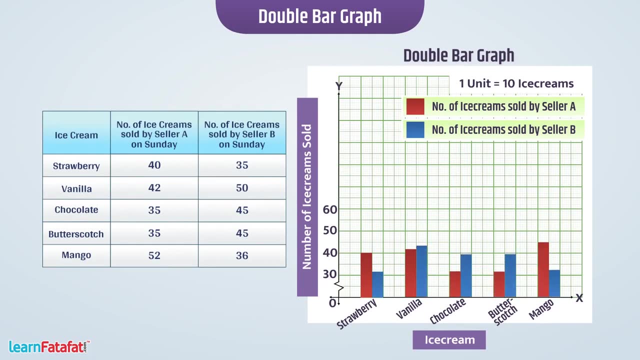 So, to represent 42, we have to consider 2 parts of unit length out of 10 parts after 40. Thus we will draw a bar extending from 0 to 42.. In the same way, we will finish drawing a double bar graph of the given data. 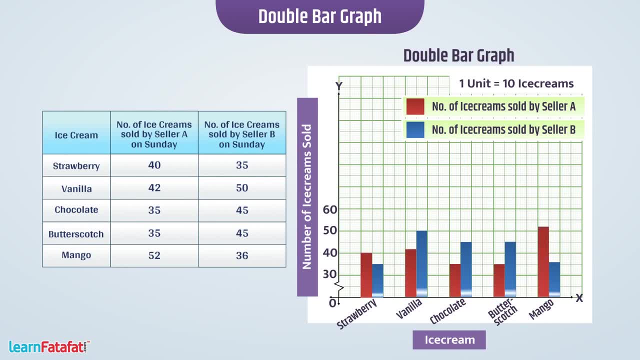 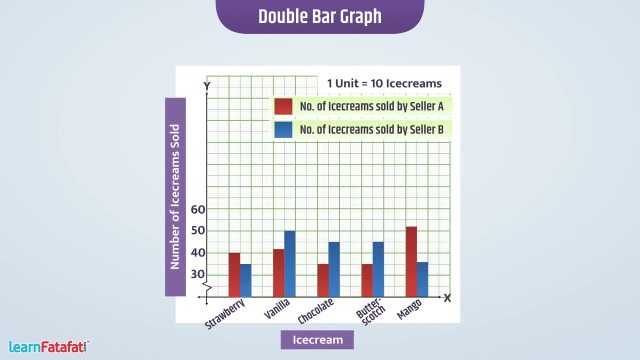 Note that we have used different kinds of bars to represent each cellar. Let's understand some of the advantages of double bar graphs. As you can see, we can easily compare the scale of ice creams by 2 cellar on the same graph. For example, cellar A sold 40 strawberry ice creams.